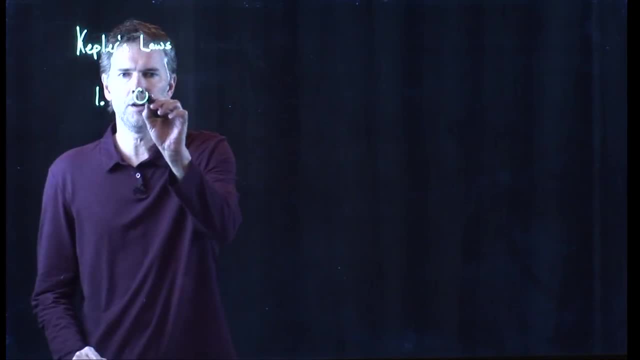 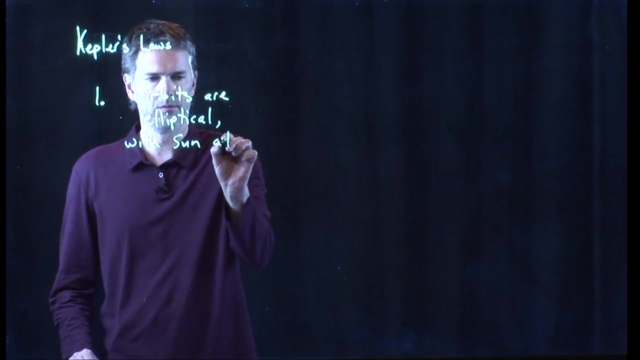 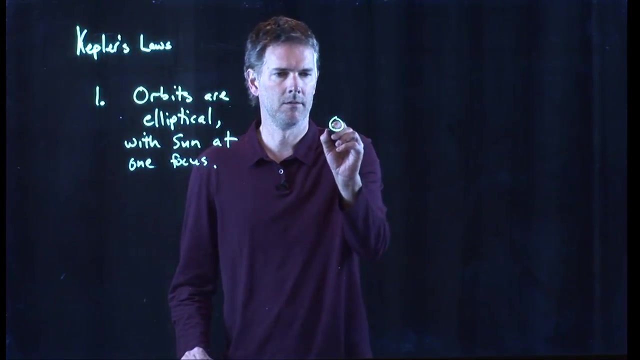 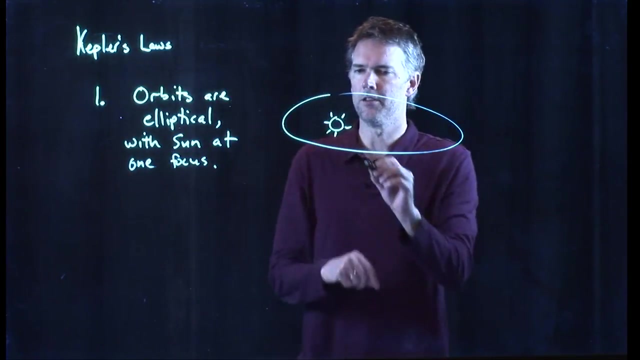 following. The first is that orbits are elliptical, And they are elliptical with the sun at one focus. Okay, so here's our sun. The planet goes around the sun, like that. The sun is at one focus of the ellipse, Okay, and an ellipse has two foci. There's one there and there's. 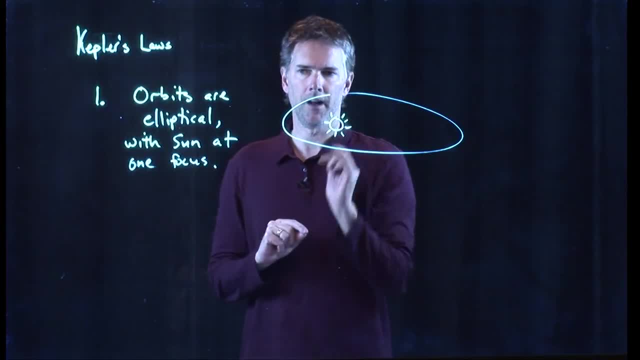 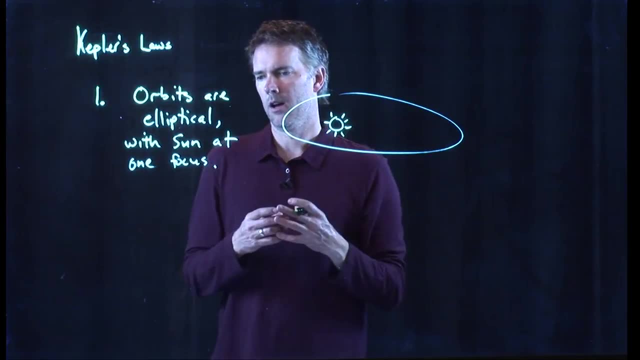 one. on the other side, by symmetry, The sun is at one of those foci. All right, This is a big step because earlier Tycho Brahe, when he came up with the idea of the ellipse, he said that the sun is at one focus of the ellipse and the ellipse. 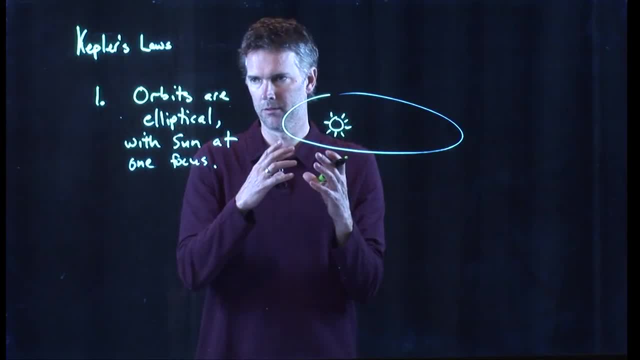 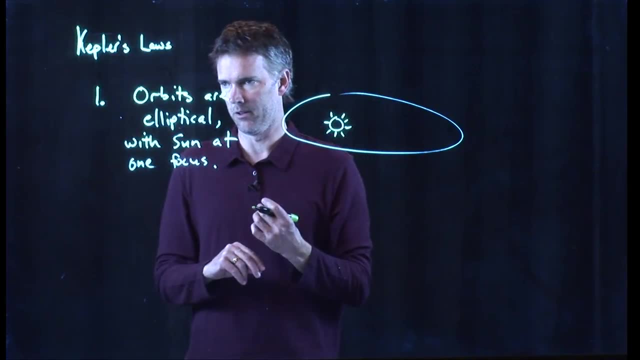 is at one focus of the ellipse Now. Tycho Brahe and other people thought that they were circular orbits, And the reason they thought they were circular orbits is because when you look at the orbit of the earth around the sun, it is nearly circular, Okay, But other planets have much more eccentric 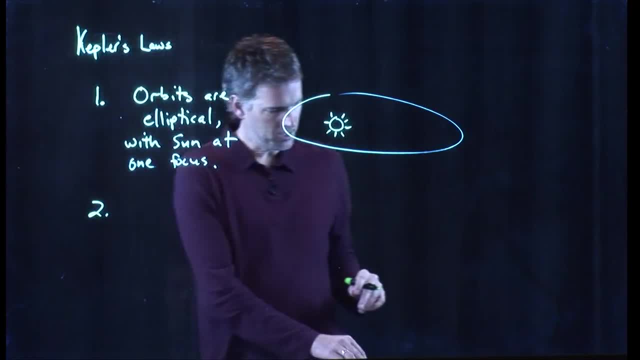 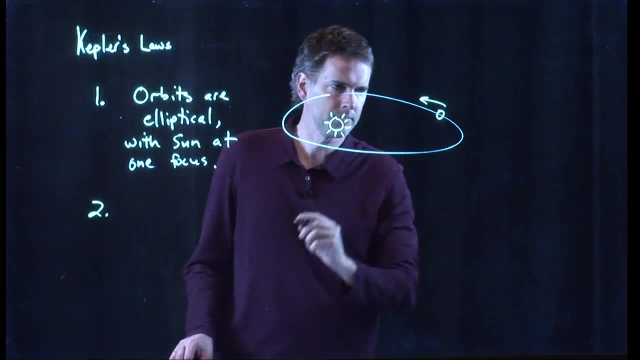 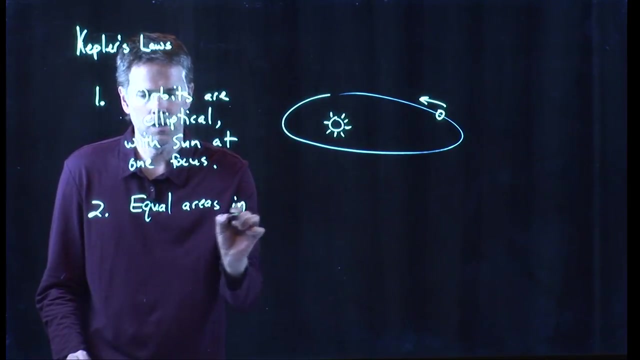 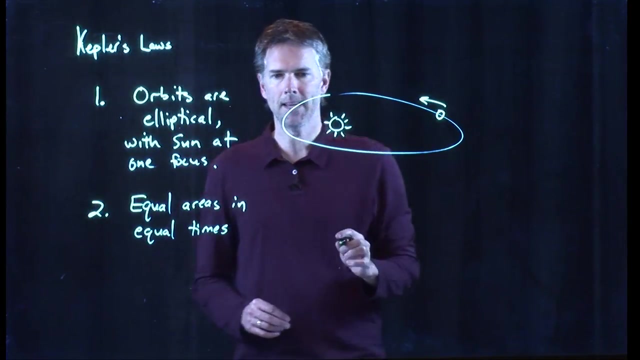 orbits, All right. The second law that he came up with was: and let's draw our planet on there, heading around. The second law was the following: Equal area, Equal areas in equal times. Okay, so what does that mean? on our picture here, What it means is: as this planet sweeps. 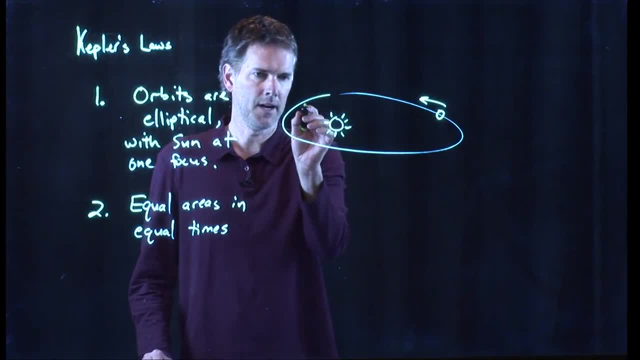 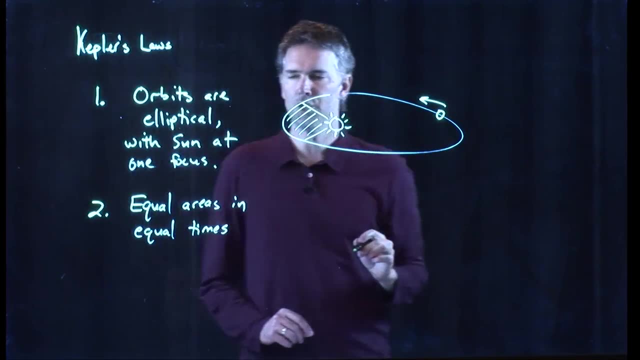 out this ellipse about the sun. if I take a stopwatch and I measure how far it moves in some amount of time and then I shade that area, I would get some number. But if I take the stopwatch and I do the same amount of time at the far end of its elliptical 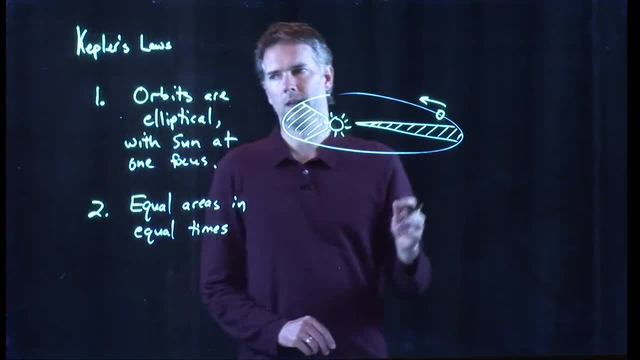 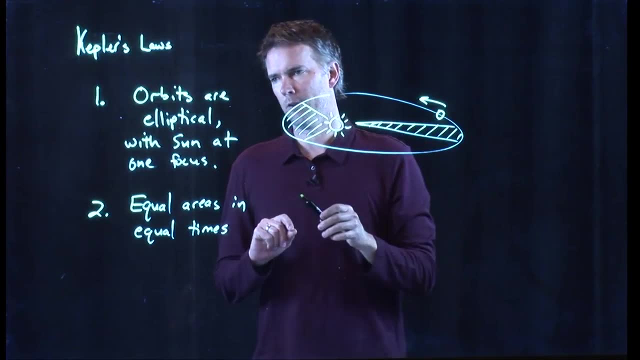 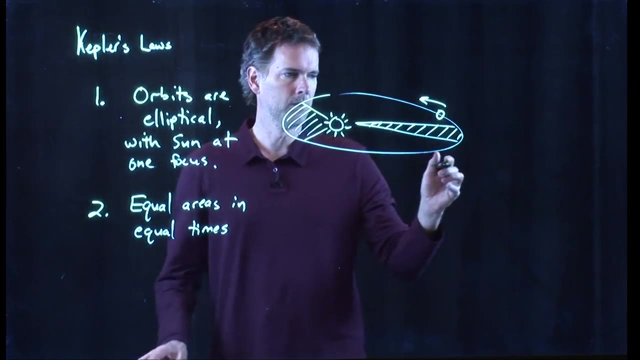 orbit and I map out that area, I get the exact same number. Equal areas in equal times. So if this is one month of an orbit, you get some number. One month of an orbit, you get the same number. This necessarily tells you that the planet is moving slowest. 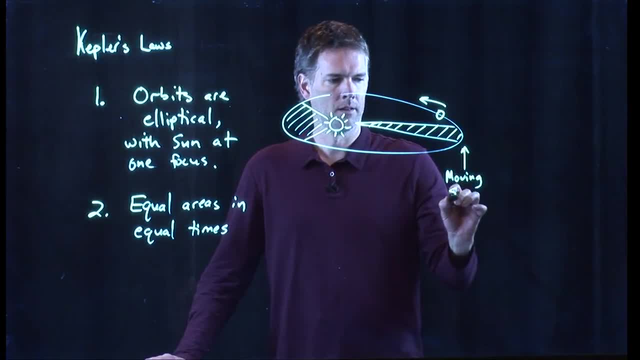 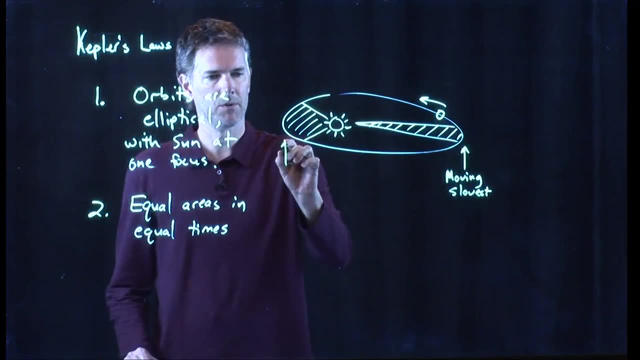 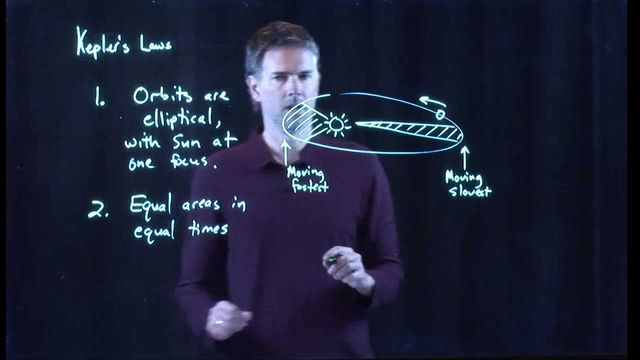 Slowest, Slowest, Slowest, Slowest, Slowest, Out here In order to get the same area as this region where it is moving fastest. Okay, planet kind of zips in towards the sun, goes back out, slows down a whole bunch. 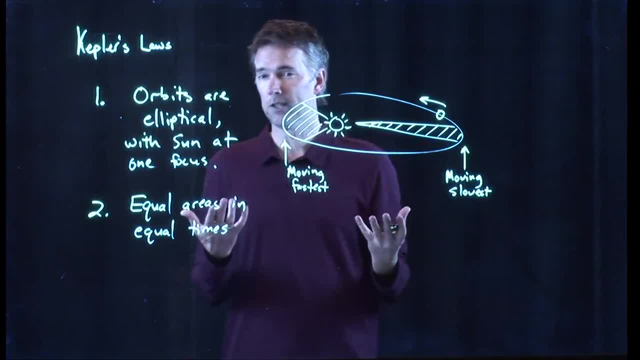 and then comes and does it again, And this is sort of like the slingshot that you guys have heard, The gravitational slingshot, Right. When an object goes past a massive object, it is moving fastest when it's closest to it and then it shoots back out. 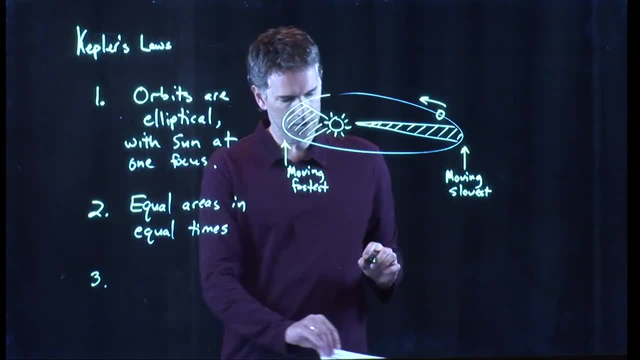 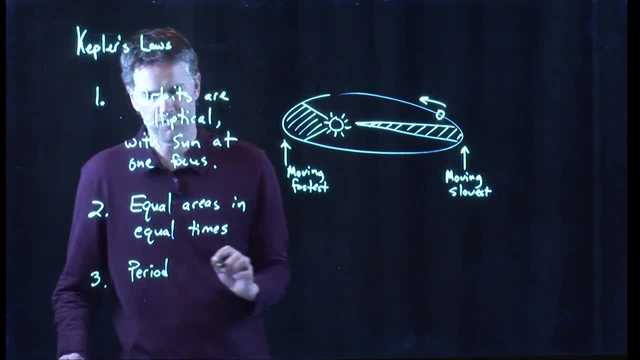 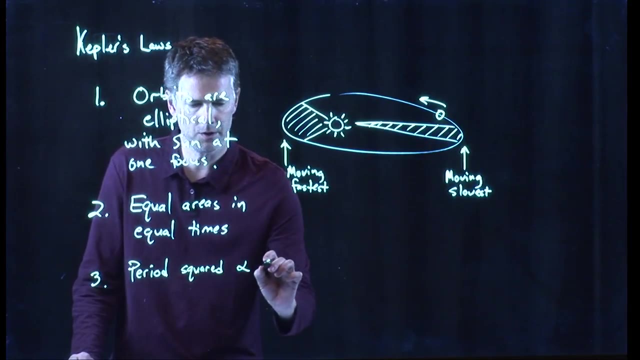 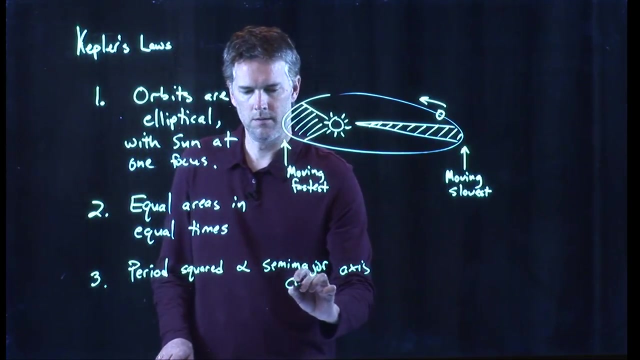 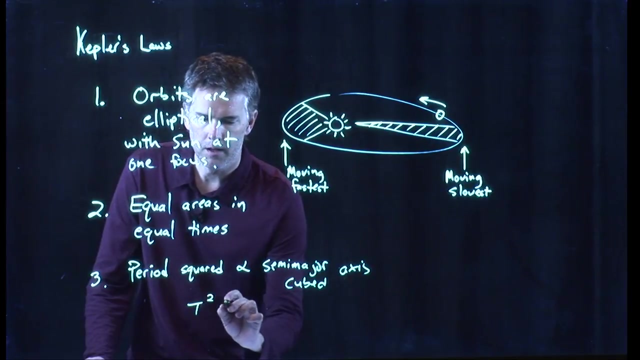 Alright. the third law that Kepler came up with, which is a little bit more difficult to see, is the following: The period squared is proportional to the semi-major axis of the elliptical orbit. Semi-major axis cubed. Okay, in words that's what it is. 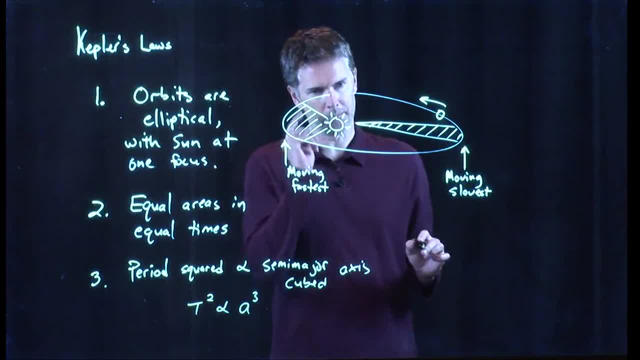 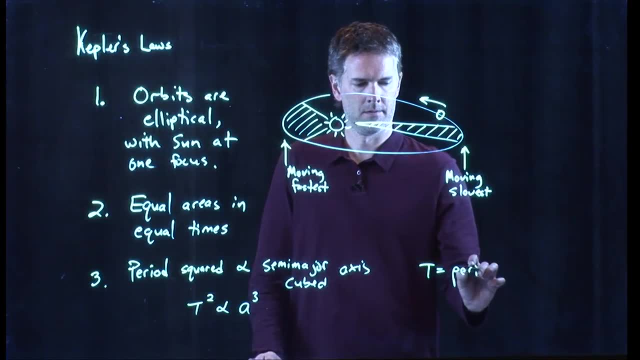 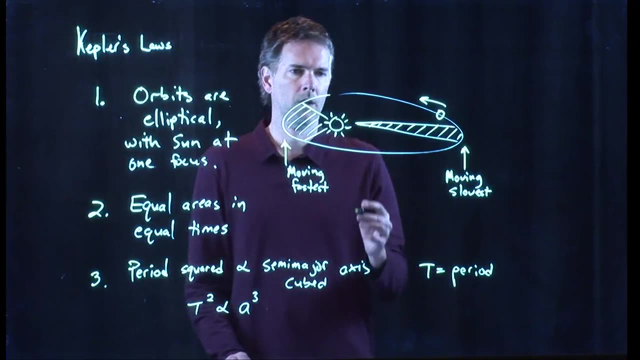 In math it looks like that T squared is proportional to A cubed. T is the period. So for the Earth the period would be one year. What is this semi-major axis cubed? Well, if I take my ellipse and I draw the bisector of that ellipse, then this is the 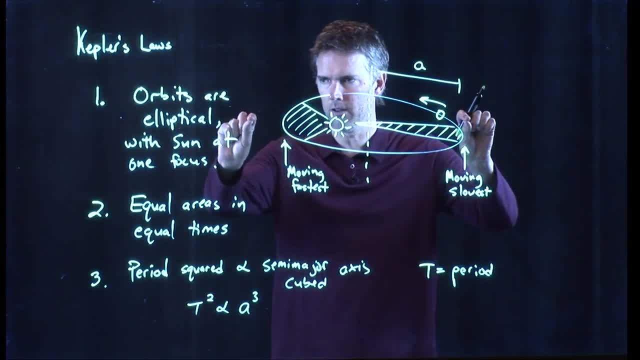 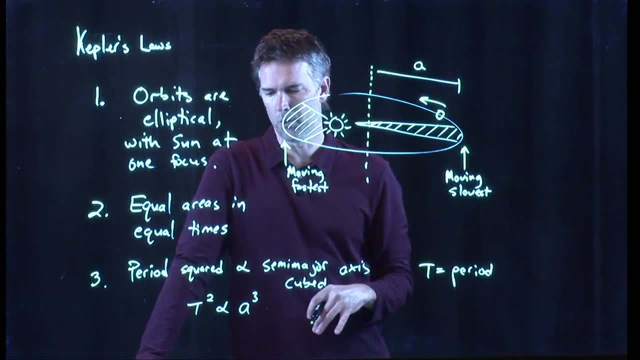 semi-major axis. The major axis is the entire length of the ellipse. The semi-major is half of that. Okay, So he found that the period squared was proportional to the semi-major axis, cubed, which was a huge step in understanding the motion of the planets. 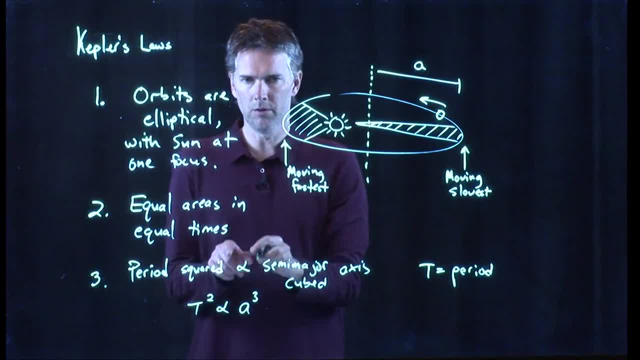 And what we're going to see is that, in fact, Newton's universal law is that Newton's universal law of gravitation that we just talked about. you can use that to derive all of these laws, All of Kepler's laws, are derivable from Newton's universal law of gravitation. 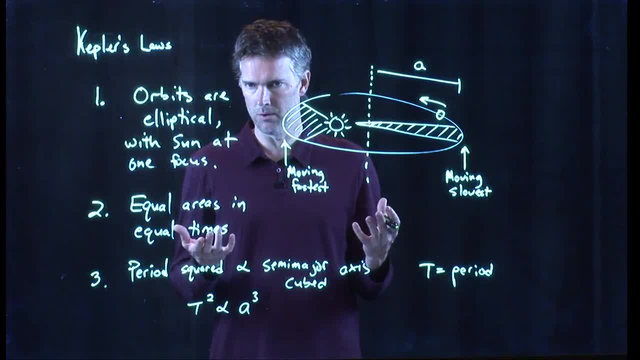 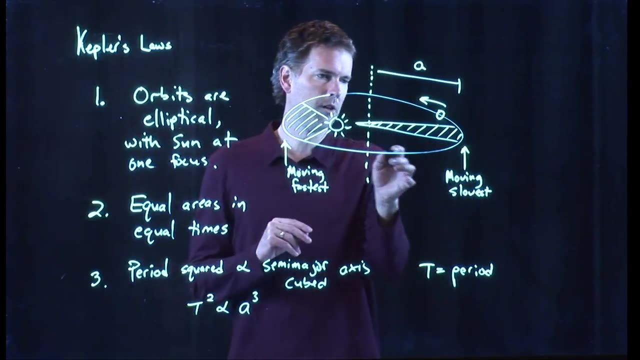 This is one of the reasons that it was such a huge step by Newton. was he sort of tied all the planets together? He tied our entire solar system together with one law, which is pretty remarkable. Okay, What we said was highly elliptical orbits are very eccentric. 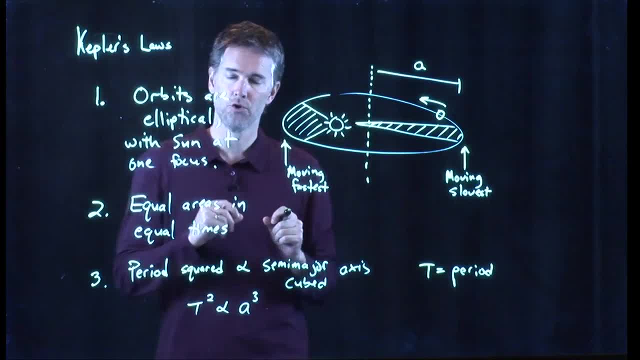 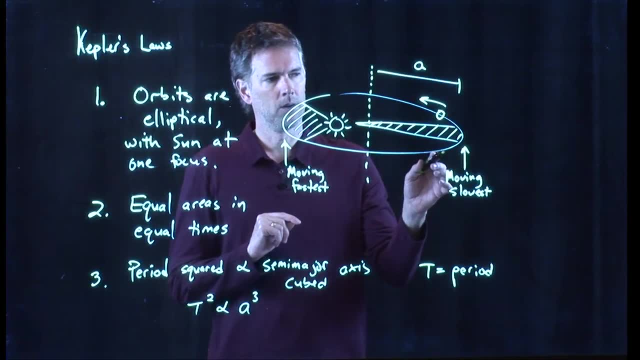 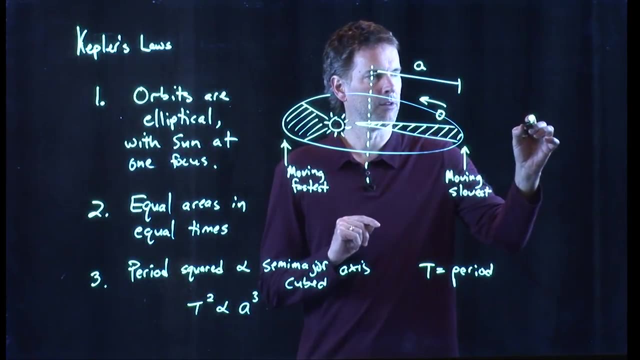 Circular orbits have low eccentricity. Okay, Usually they talk about an eccentricity of one. So if I think about orbits that are reasonably circular, that would be stuff like the Earth. So if this is our Sun, the Earth has an orbit that looks like this: 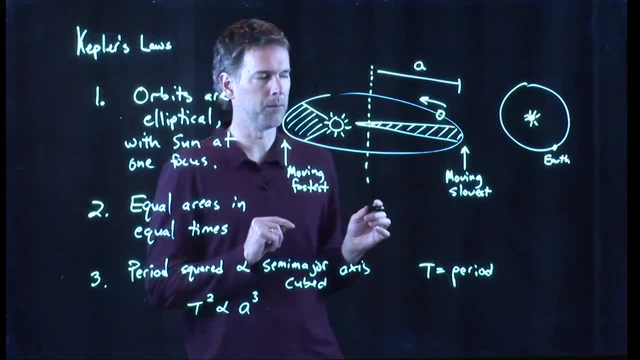 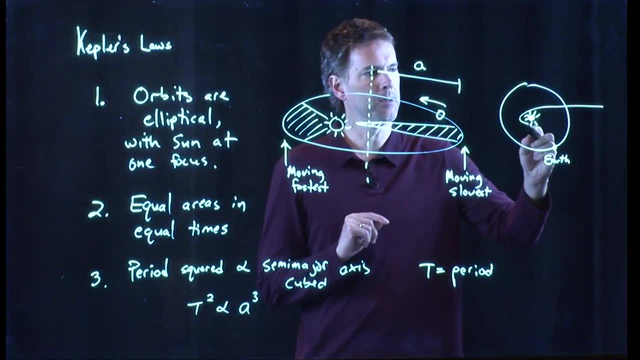 Nearly circular. okay, It's still elliptical, but it's nearly circular, Whereas Halley's Comet comes in very steep and shoots way back out. This might be something like Halley's Comet, And Halley's Comet has a long period right. 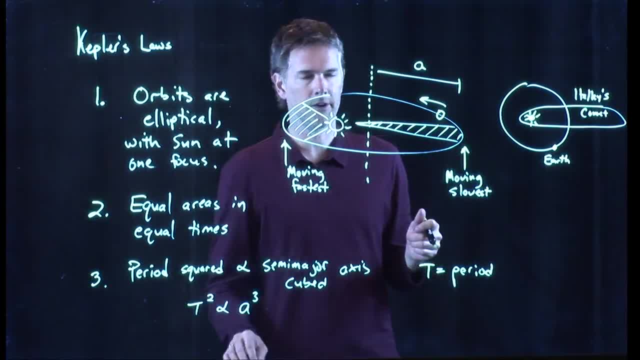 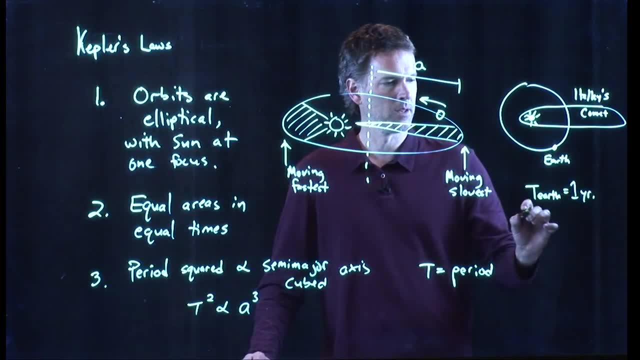 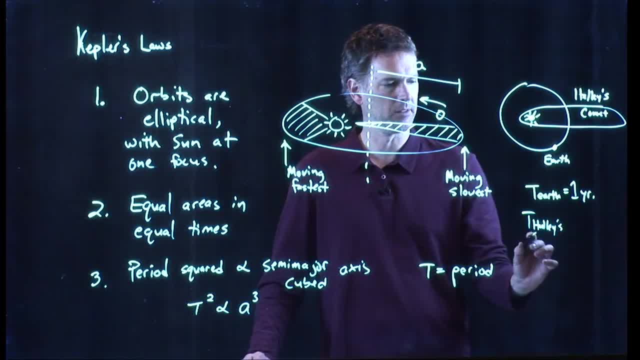 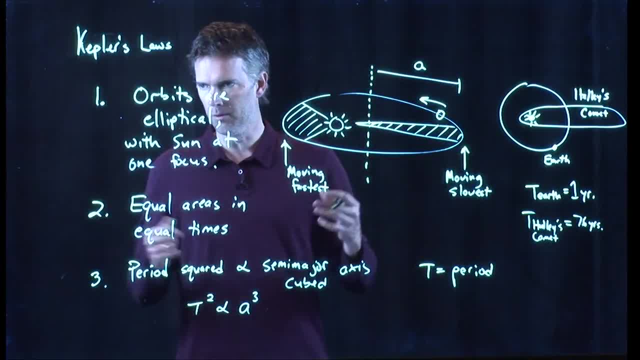 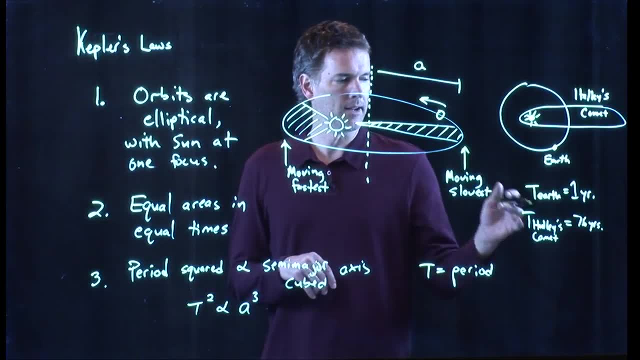 It is about 76 years. Okay, So we're going to see it again in 2060.. You guys will likely be around to take a look for Halley's Comet in 2060-something And definitely try to catch that with your telescope if you're around. 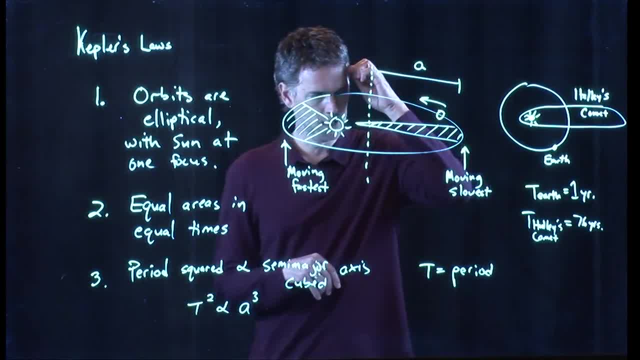 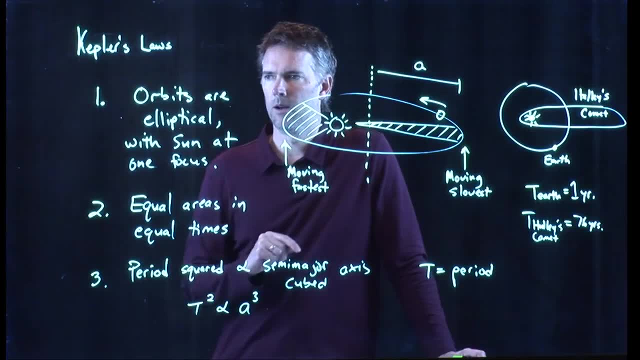 It's a really nice sight to see, to see. I saw it back in the 80s and in fact my grandfather, who was alive at the time, he looked at it with me when Haley's comic came by and he said, oh yeah, there it is again. and I said: what he goes? yeah, I saw it when I was 8 years. 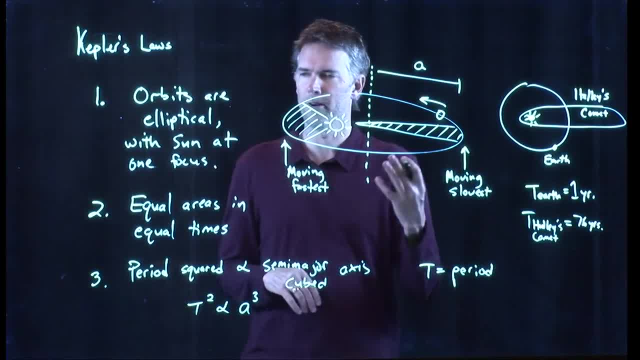 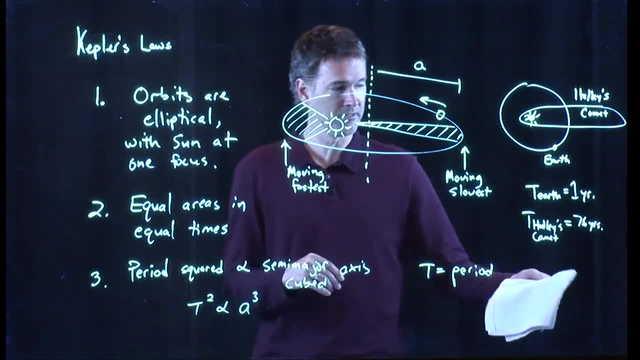 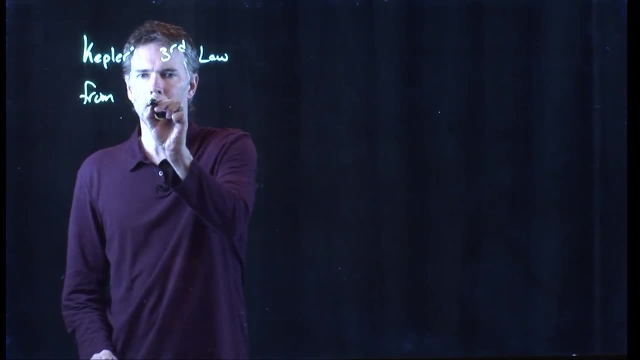 old standing in the fields in Montana. I just looked up and there it was. and now it is, 76 years later. it's here again. so kind of rare that you would get to see it twice in your lifetime, but it happens. okay, let's see how Kepler's third law is. 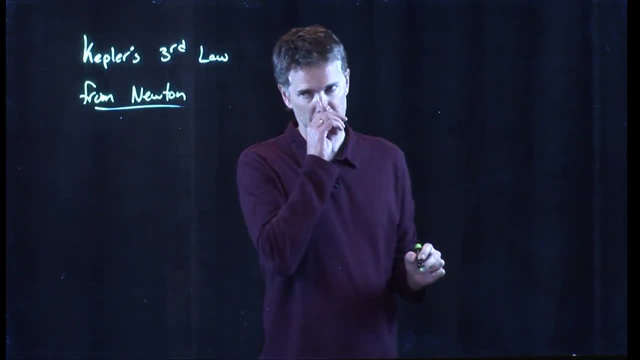 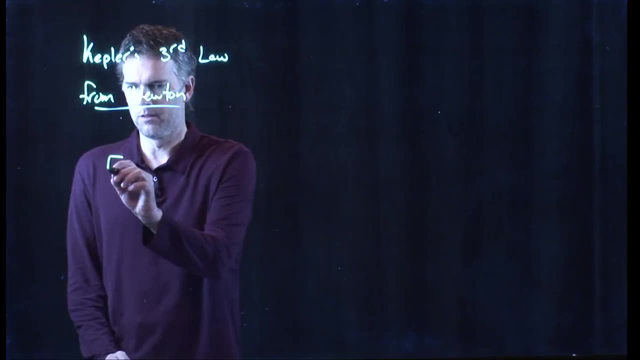 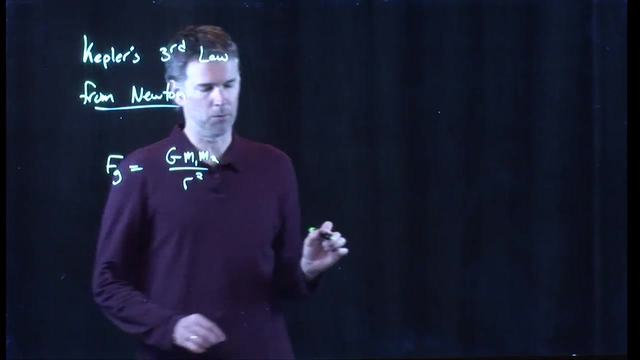 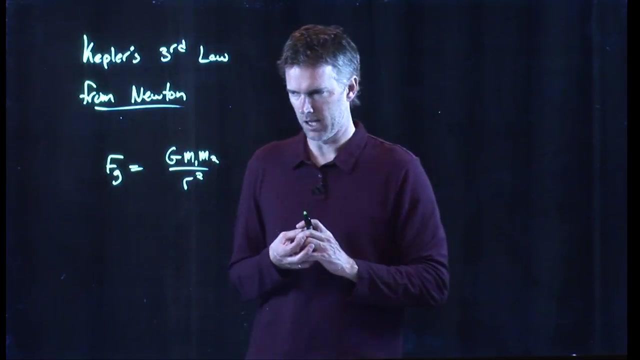 derivable from what Newton said. okay, so Newton said the following: the force of gravity, the magnitude of it is G, m1, m2 over R squared. any two masses are gravitationally attracted to together by that magnitude. okay, usually we put a minus sign in front of it, but 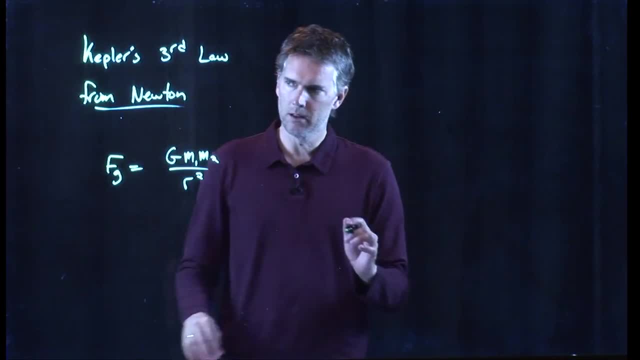 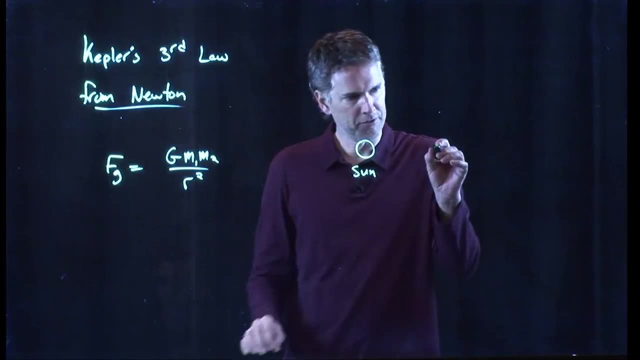 this just means it's attractive. so let's take the. let's take the example of a planet orbiting the Sun and let's put it in a circular orbit. so the Sun has mass M sub s, the planet has mass M sub P, and now this thing's going to go about the. 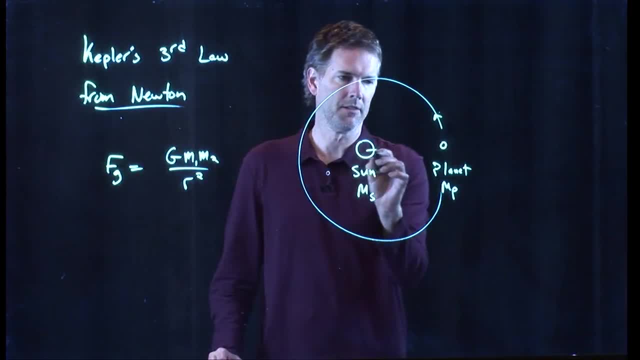 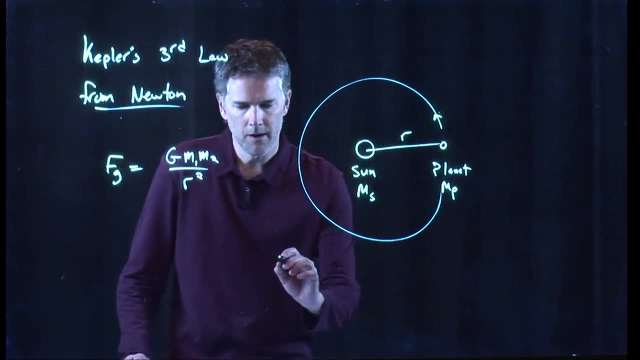 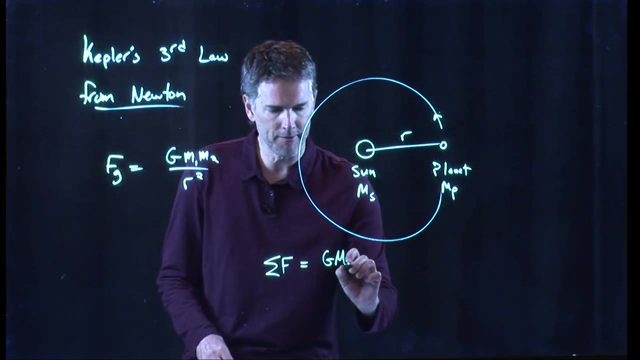 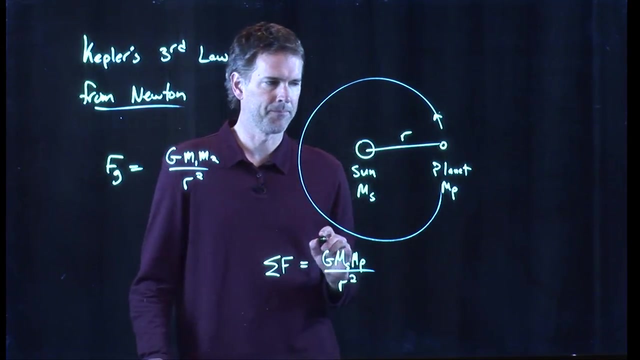 Sun in a circular orbit. it's a distance r from the Sun. What do we know? What we know is there has to be a force on that planet to keep it moving in a circle. That force is just gravity, and so it's g mass of the Sun, mass of the planet divided by r squared. But we 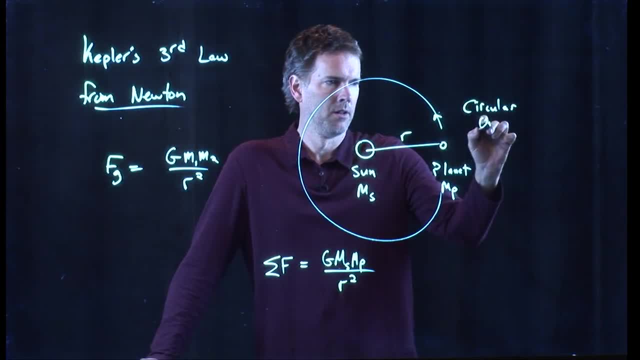 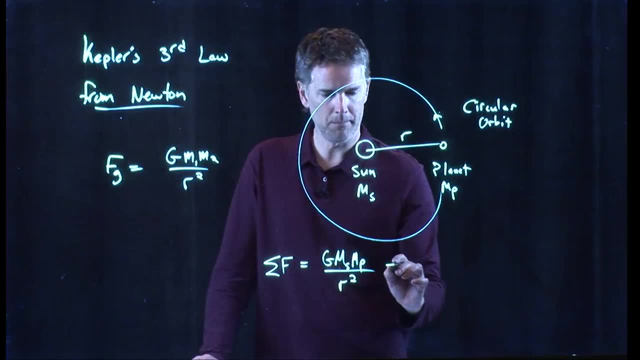 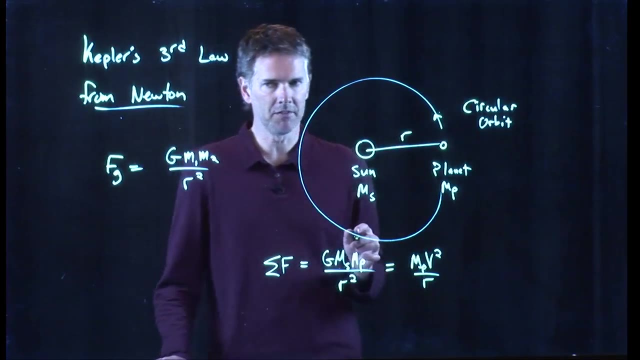 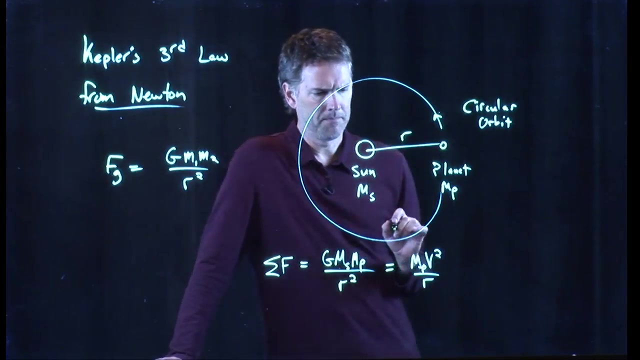 know if this thing is moving in a circle. those forces don't add up to zero, They add up to something else. What do they add up to? mv squared over r, Okay, and the m in this case is the mass of the planet. All right, that looks pretty good, but we 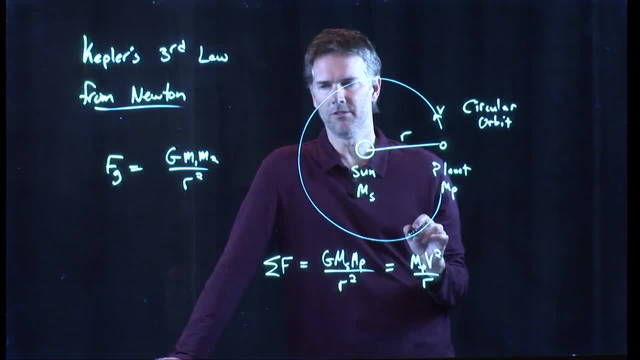 don't know exactly what v is Right. v is the speed of this thing. Okay, so we don't know exactly what v is Right. v is the speed of this thing. So we don't know exactly what v is Right. v is the speed of this thing. 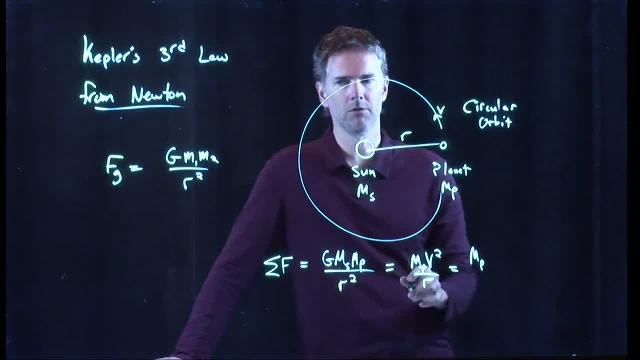 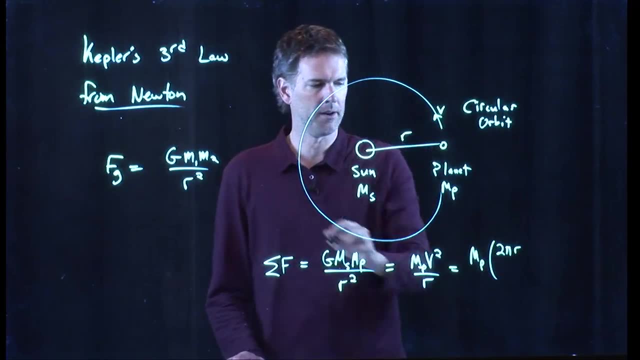 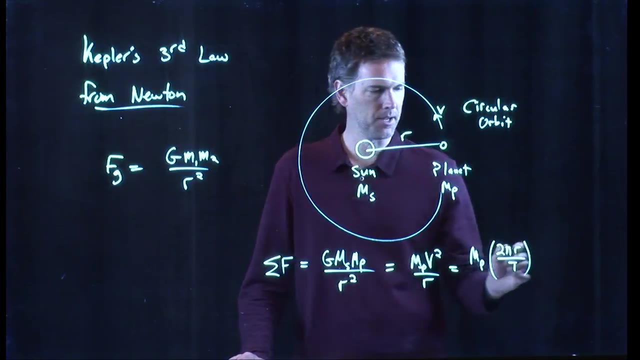 But what we do know is that if it goes all the way around, it goes a distance 2 pi r, And if it goes all the way around in an amount of time, t, then that speed is just 2 pi r over t, distance, over time, And that thing. we got a square and we still have an r in. 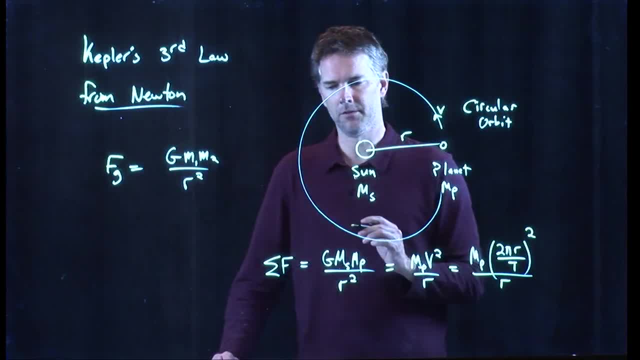 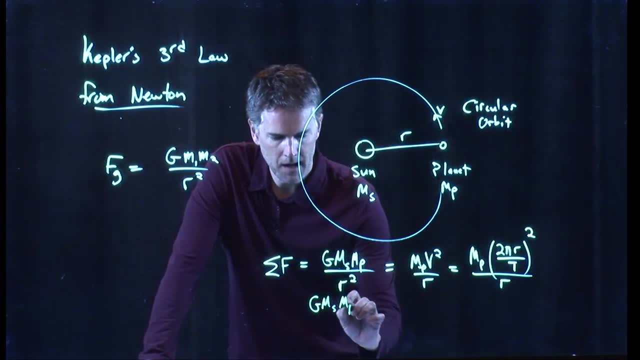 the bottom. Okay, and now we can simplify this quite a bit. What do we get? We've got g, m sub s, m sub p, over r squared equals. let's multiply this stuff out. We've got a 4 pi squared, r squared. we have an r in the bottom, and then we end up with a capital T squared. 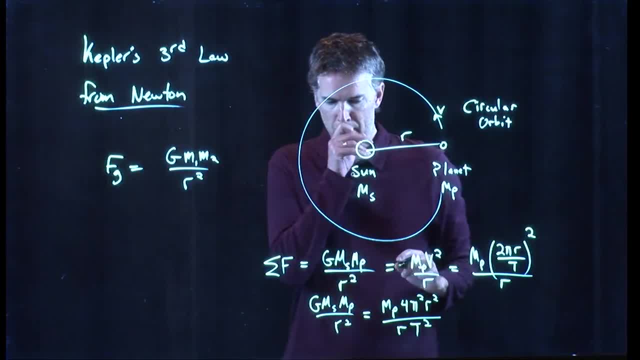 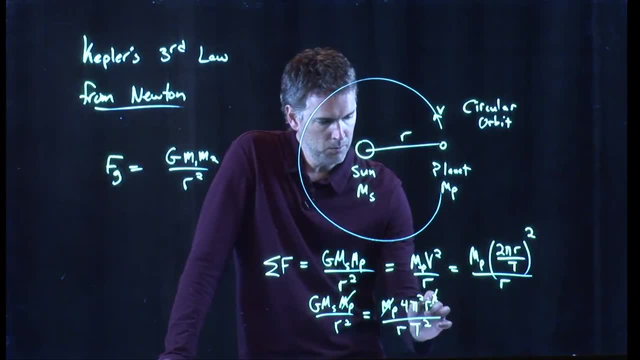 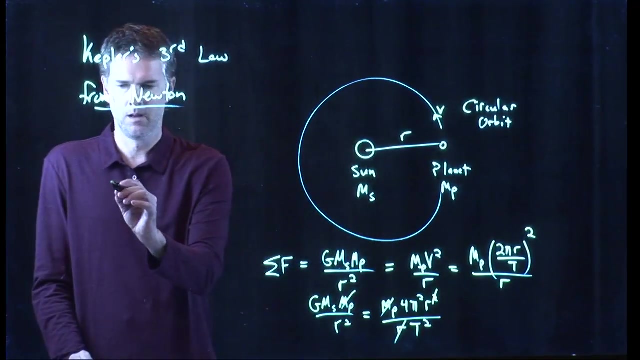 in the bottom. Okay, and now we can cross out some stuff. mp drops out. If I cancel one of these r's, I can do that, And if I multiply across by r cubed, I can write a very nice formula which is the following: T squared- let's multiply T squared up over there- equals. 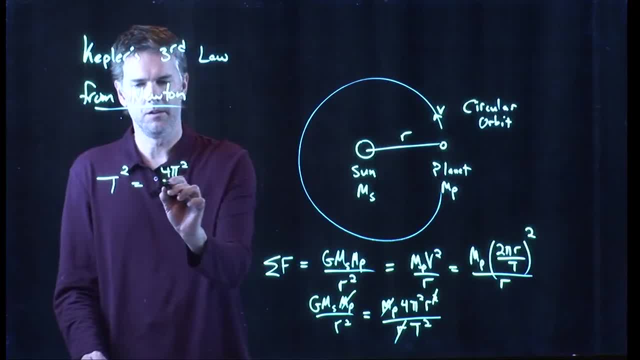 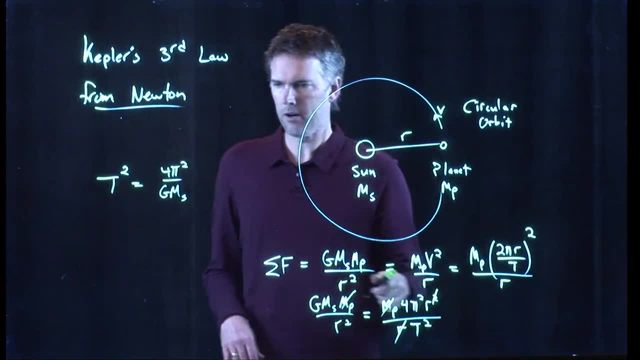 4 pi squared divided by g m sub s, And then I've got to multiply r squared up over there, so I've got a 4 pi squared divided by g m sub s, And then I've got to multiply r squared up over there, so I've 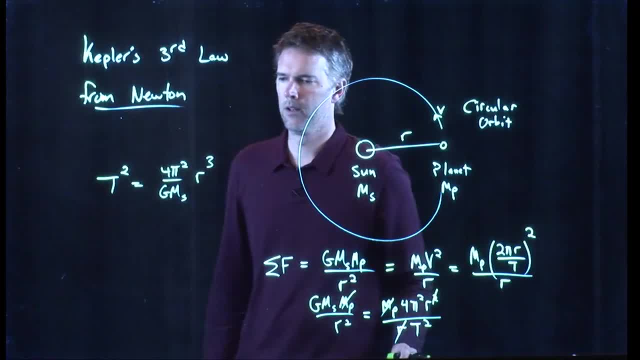 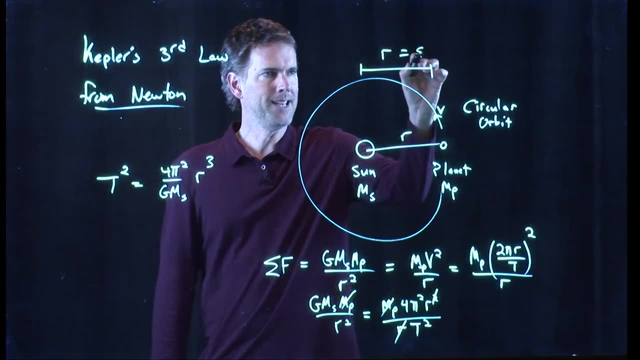 got to multiply r squared up over there. so I've got to multiply r squared up over there, so I end up with r cubed. But here's the deal, right. A circular orbit means that r is in fact the semi-major axis. 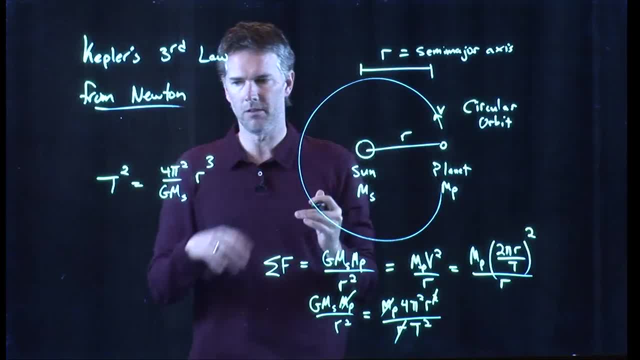 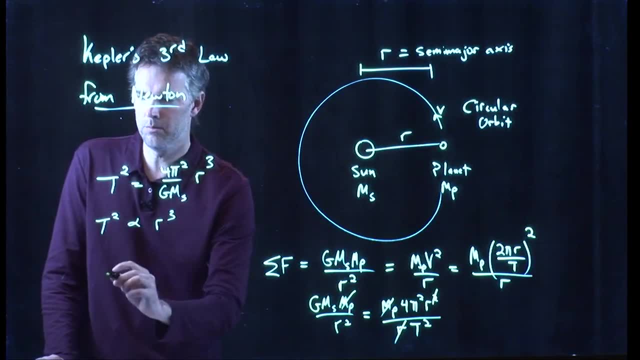 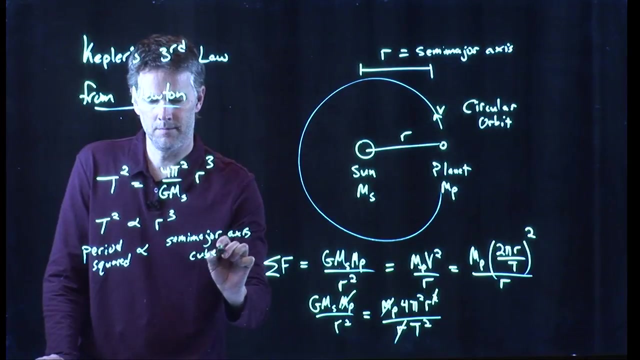 The major axis would be the diameter. The radius is the semi-major axis, And so we get T squared proportional to r, cubed, which is exactly what Kepler said. But the period squared is proportional to the semi-major axis cubed, And in fact we can write down: 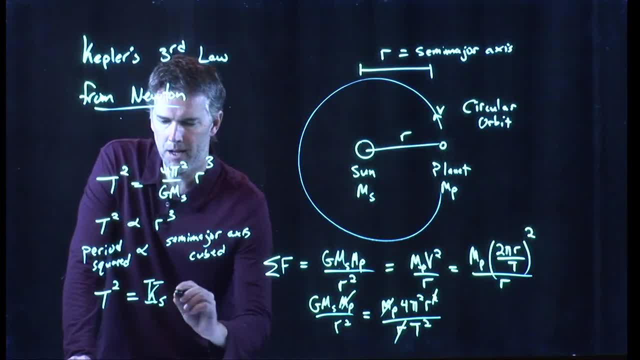 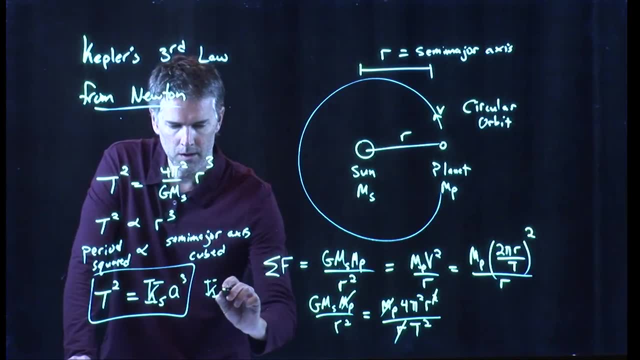 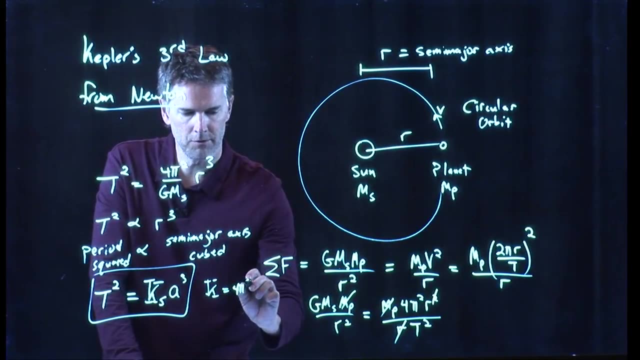 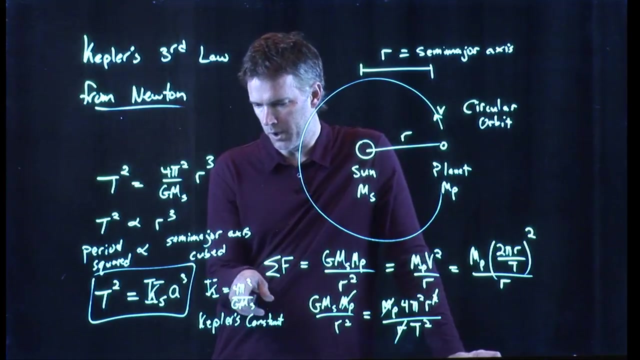 the following: It's equal to k sub s times a cubed, where k sub s is called the Kepler constant, and it has a value of 4 pi squared divided by g m sub s. This is Kepler's constant. We know the mass of the sun, we know big G, we obviously know 4 and pi, and so we can.